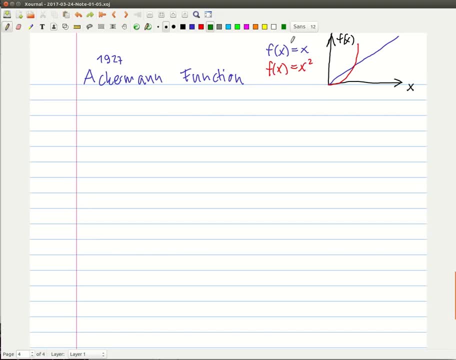 But we are not considering this right now. But it is important to know that the Ackermann's function even grows much more faster than all the exponentials and x squared and stuff, Even for small arguments. I will demonstrate it later. First let's look at the definition. 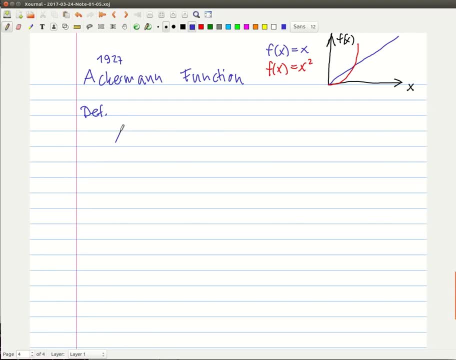 Of the Ackermann's function. Ackermann's function is represented as an A Ackermann of n, n, m Is defined as, But first I want to point out which values these arguments can take. So n and m must be an element of the natural numbers. 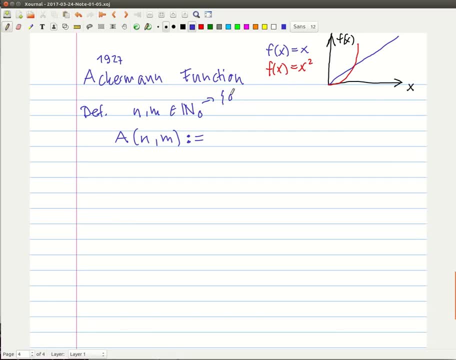 Including the zero, which is just Zero One, Two, Three, Blah, blah, blah. So You can't plug in negative numbers here, Or even fractions, Pi Or stuff. Okay, So we are restricted to positive natural numbers. 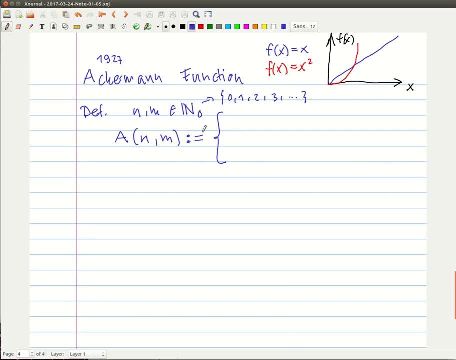 Okay, So you can see. this Ackermann's function is not a simple function like this, So you can't just write it in one line. It's kind of like a distribution. So There is Three possibilities For this function. So the first case is: 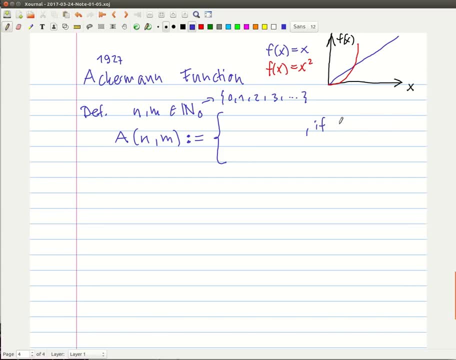 If n is equal to zero, If n is equal to zero, If we plug in a zero over here, This function will just return m plus one, Which is pretty simple. So you just have to increment This argument: m. The second one. 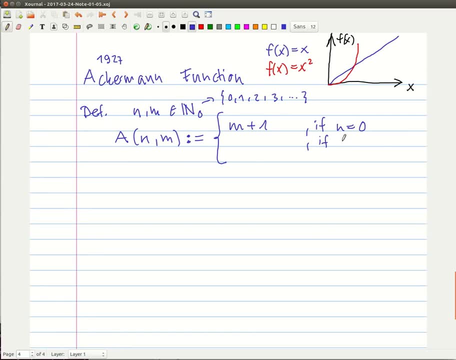 A little bit more tricky Is if m is equal to zero, And in this case We have to Recall The function. But You have to subtract a one from the first argument And Simply plug in a one Into the second argument. 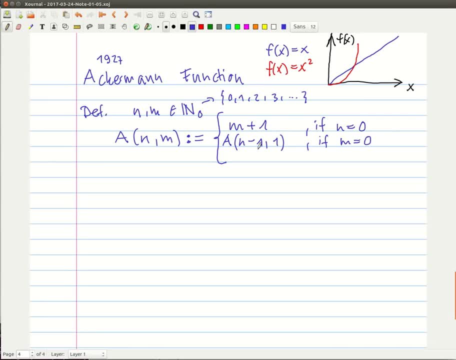 So This M, If we are in this case, Here is a zero And here is Any Any number, So it can't be zero, But The number Will be changed to a one. That's A pretty easy operation. 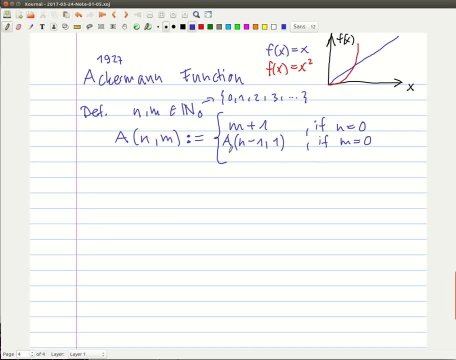 So this is not Too Bad looking, Even though It's a recursive call And The last case If Those Statements aren't true. This is The more Ugly looking Thing And minus one. And then you have. 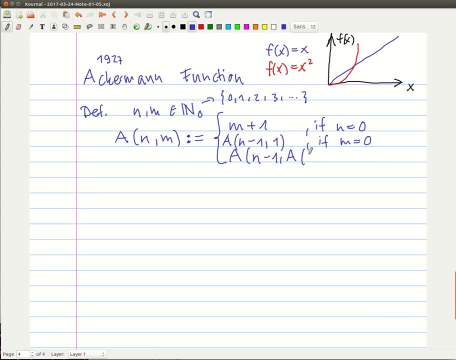 In the argument You have a recursive call Of the arguments function again And minus one Else. Okay, So Yeah, Let's try. Let's try to To see how we, How we, We solve that. First of all, 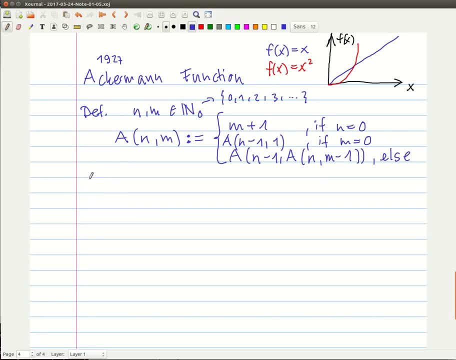 I would consider A Case Like A Case of zero Comma Five. Excuse me, What is that? Well, R, N Is equal to zero, M Is equal to five. So This case. 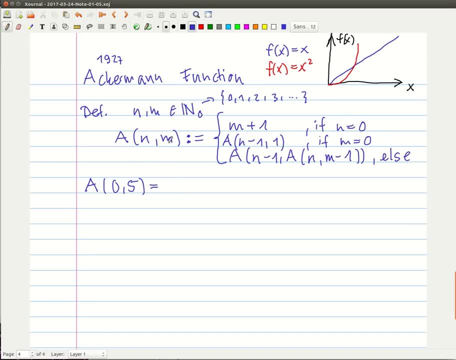 Shoots. That is our case. We don't have to Worry about These guys Here, So This Case Should. So That is our case, We don't have to. So M Is equal to five. 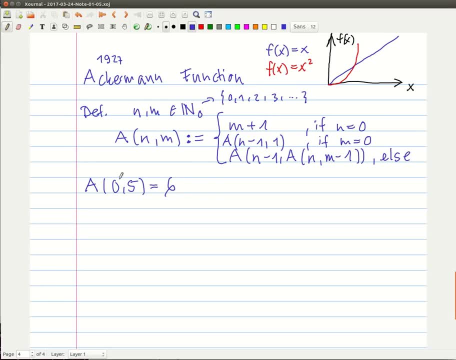 Five plus one Is six, So That was easy. If you Have an Ackermann Function of zero Comma- Something You Always have The result Immediately. Okay, Let's Try something More Tricky. 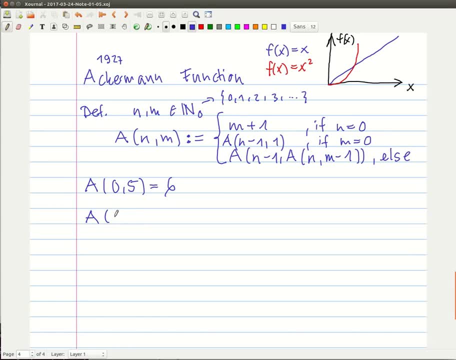 Like Ackermann, Of It's Not Making Too Complicated. Well, This Is Equal To Well, Okay. Or N Is Equal To One And Or M. 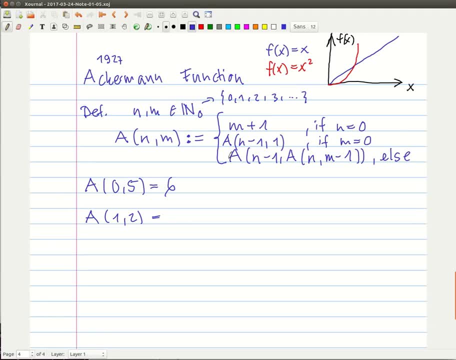 Is Equal To Two, So These Two Cases Don't Hold Okay, So We Have To Plug This N At This One. Sorry, Into Here Which. 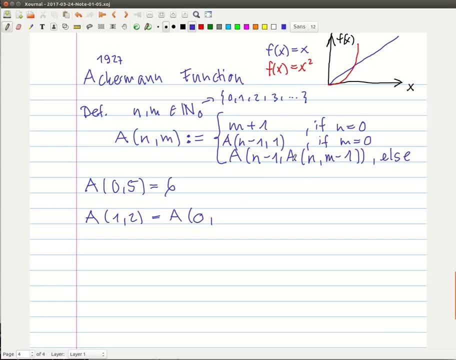 Will One Minus One, Which Will Give A Zero, Here And Now, In The Second Argument Of The First, By One. So M Is Equal. 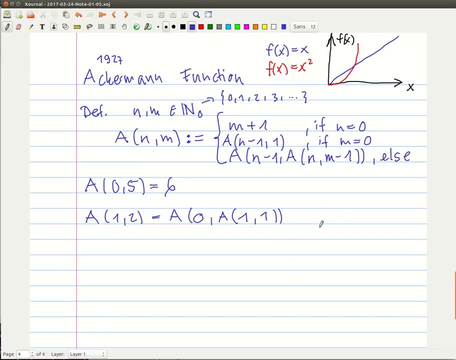 To This Will Yield One Over. Here And Now. You Might Ask: Well, What Did We Gain, Since We Still, We Still Have These Arguments? Well, 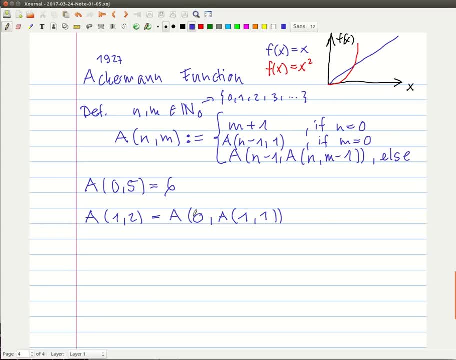 Maybe You Realize That This Argument Decreased And Also This Argument Decreased, And We Might Be Able To Run Into A Case Such That. 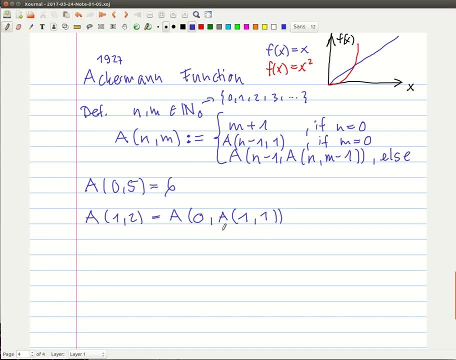 M Is Equal To This And Let's Look At It And I Think It's It's Easier To Understand That Doing It In The Way 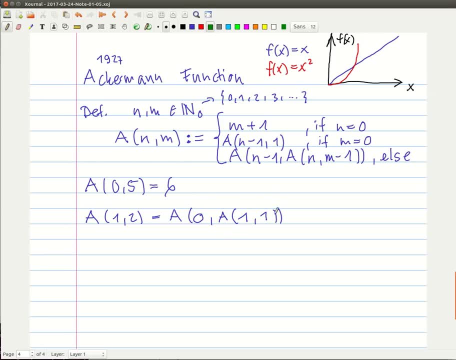 I'll Show You Right Now. Okay, So We Just Concentrate On Computing This And, As You Will See It, Basically It's Very Easy, It's. 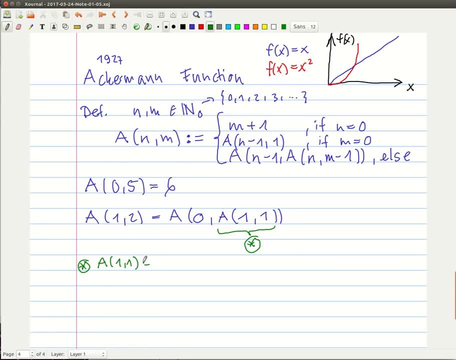 Just A Lot Of Writing And Substituting. Okay, We Just Want To Compute The This Ugly Looking Thing Over Here But Our N Here. 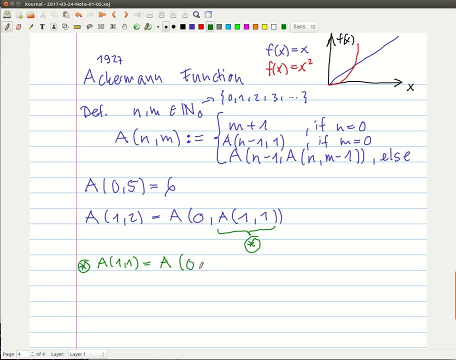 Is Equal To One And We Have To Subtract The One, Which Will Give A Zero. Nice Okay. Another Function: Decrease The M By One. 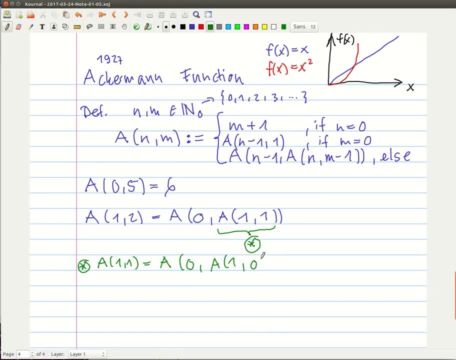 So Which Will Yield Zero? Okay, And Now Let's Look At This Body Here, Which Is A Command One. Now Realize That Here We Have. 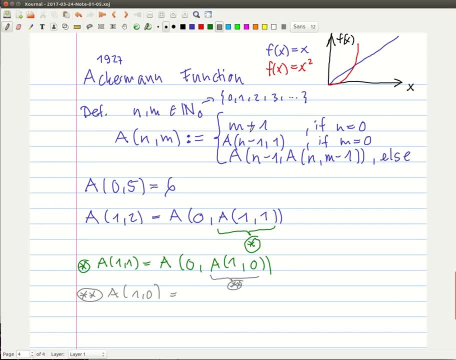 A Zero. So Our This Function, Or Better Say This Function Or M, Is Zero. So We Have To Look At This. But What Do We? 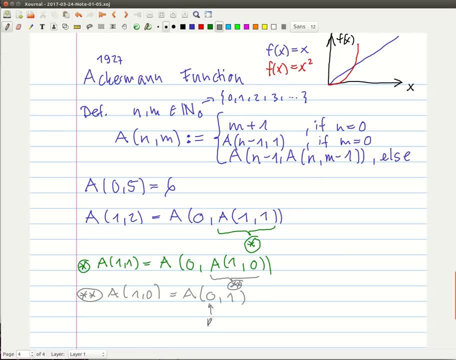 Have Here Now. Remember: This Is The N, This Is The M And Our N Is Equal To Zero, So We Can Apply This One Here. 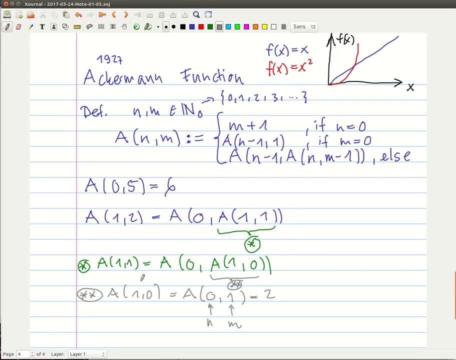 And We Can Simply Resubstitute This Into This Guy Here. So We Have Just Computed This So That Means This Is A Zero Comma. 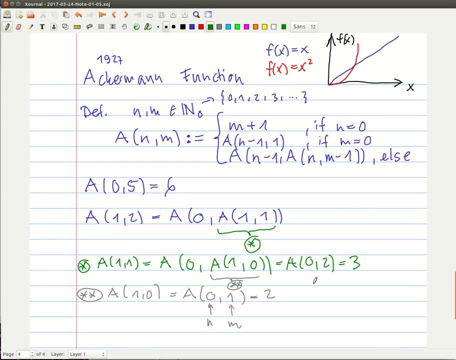 Two, What Is It Okay Here? Substituted Into Here Um Is Equal To A Sub Zero Comma. Uh, Three, What Is That Okay We? 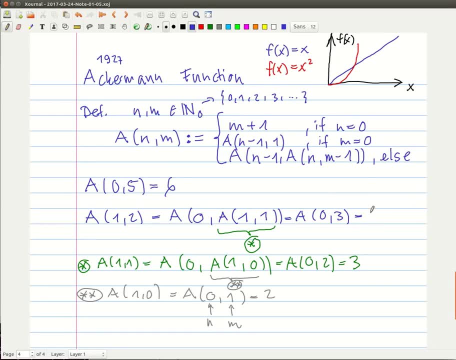 Have A Zero Here. Good Shape M Is Equal Three Incremented. I Mean You Can Compute The Functions For Little Larger Values Than This One. 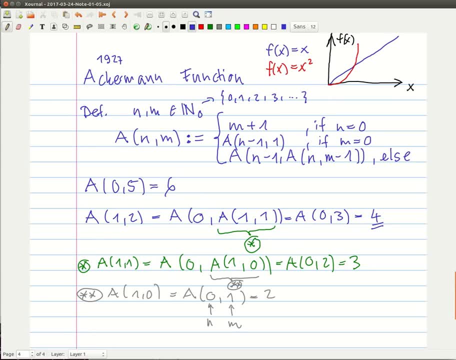 You Can Check It On Wolfram Alpha, What You Want To, But I Would Not Compute This One. You Can Also Theoretically, Theoretically. 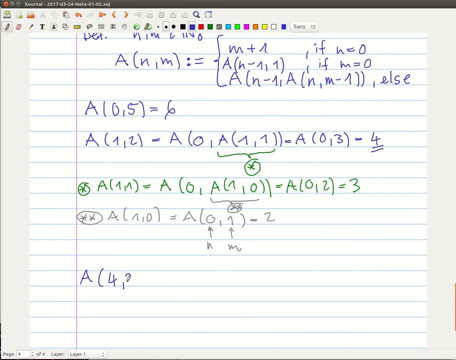 You Can Compute A Common Four Comma Two, But I Would Not Do It By Hand, Since You Need A Lot Of Things You Can. 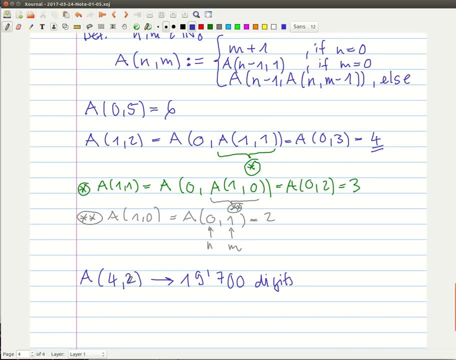 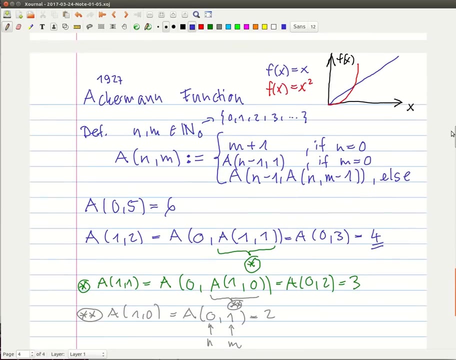 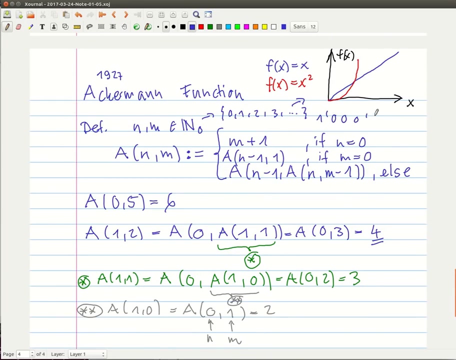 Check It How It Can Get A Number Of Things You Can Take A Part Of Things. So You, As A Part Of Things You Can. 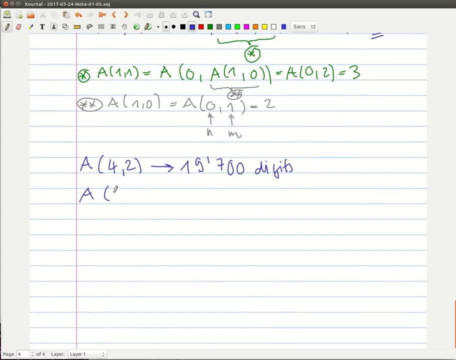 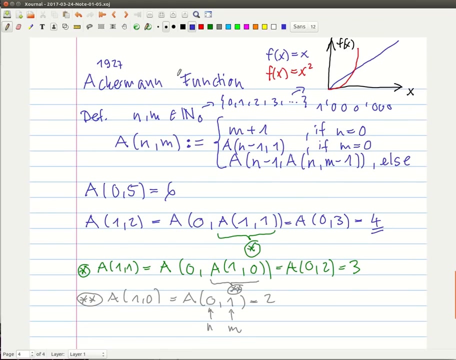 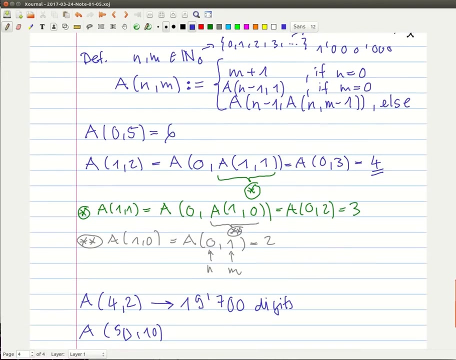 And I mean even if you plug in a 5010, I mean whoa, this thing will explode. you know- And I think Ackermann used this definition to determine whether things can be computed or not- I mean, for a computer this function can pose a big problem, or it's just very challenging to deal with very large numbers. 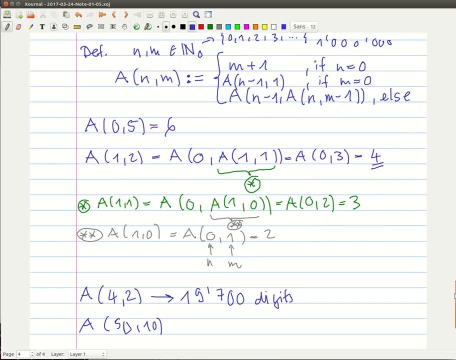 It can be Okay. well, that's it. I hope you learned something about the Ackermann's function.